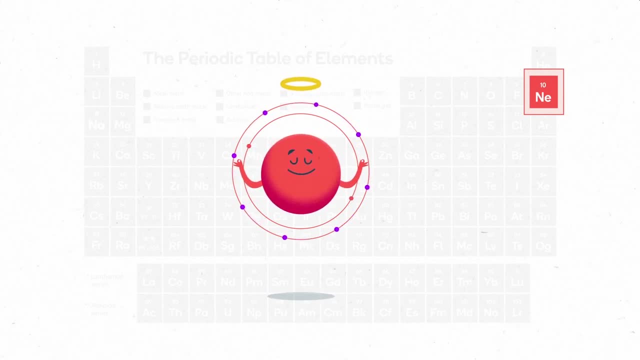 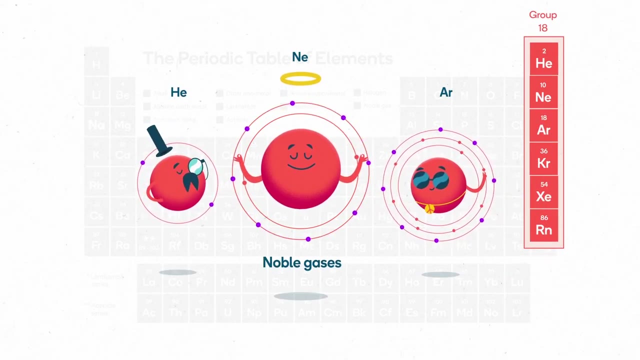 Since neon has this, it doesn't need to react with other atoms. It's satisfied all by itself. Neon and the other elements in group 18 of the periodic table are known as the noble gases. They all have a full outer shell of 8 valence electrons. 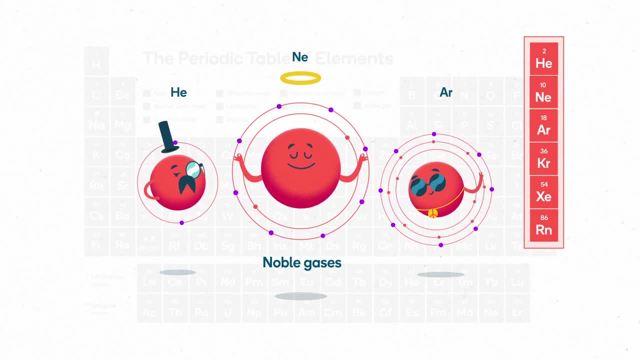 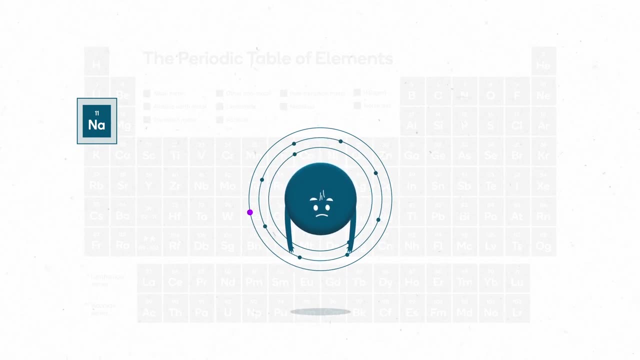 or two in the case of helium, and this makes them unreactive. In contrast to neon, sodium has one electron sitting in a valence shell all by itself. According to the rule of thumb. it wants to have a full valence shell. 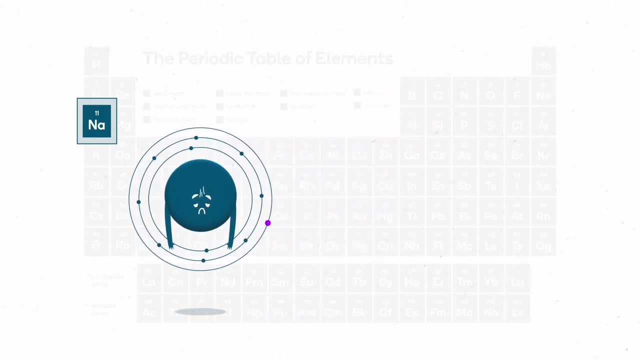 so this lonely valence electron won't do. A sodium atom can get rid of this electron by a chemical reaction. Until they are relaxed, the atom won't react with energy. Atoms react and form bonds by either sharing or transferring valence electrons. 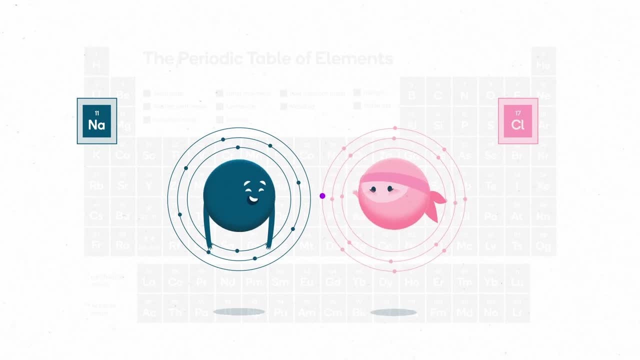 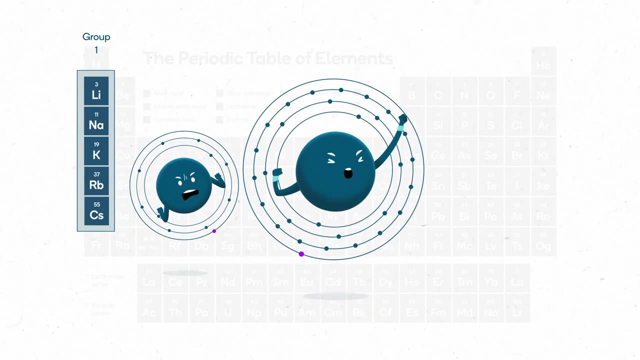 For example, sodium, can transfer its electron to a chlorine atom and they can react to form a happy couple. table salt, Sodium and the other elements in group one of the periodic table are known as the alkali metals. They all have one valence: electron. 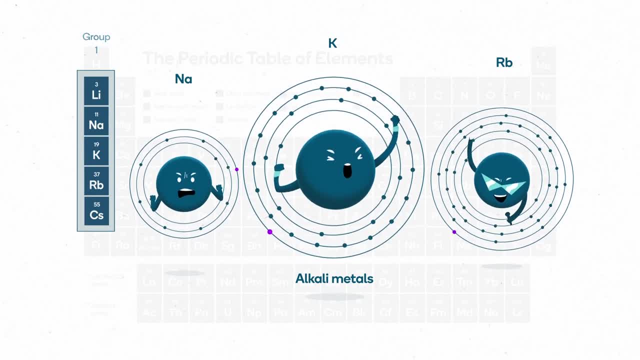 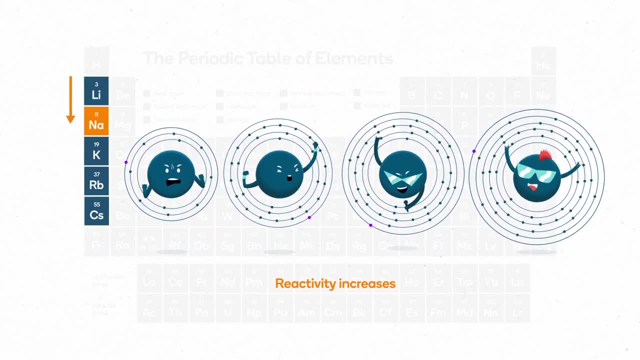 that can be transferred in a reaction. This makes them all highly reactive with substances like water, oxygen and acids. But we also observe that reactivity increases as we move down group one. For example, cesium is much more reactive than sodium. 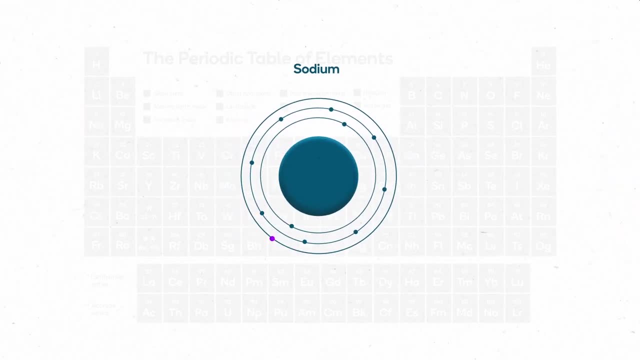 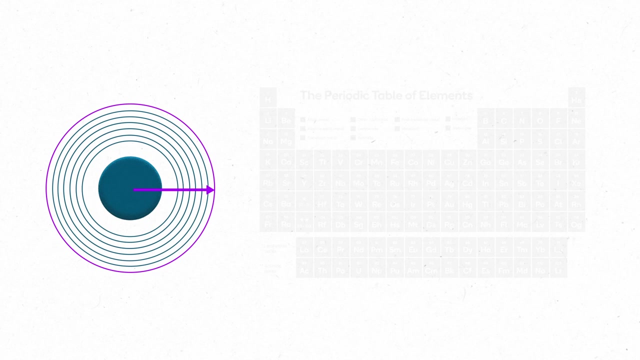 Why? Well, it has to do with the size of the atoms. The distance from the center of the nucleus to the outer shell is called the atomic radius. Atomic radius increases down each group in the periodic table as each electron shell is filled. For example, lithium has two shells. 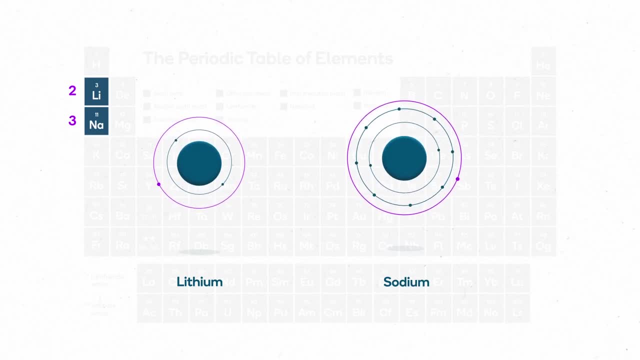 containing electrons, while sodium has three Sodium's valence shell is further from the nucleus, so it has a larger atomic radius. This explains why sodium is more reactive than lithium. Come at me, bro. Electrons orbit the nucleus because they're attracted. 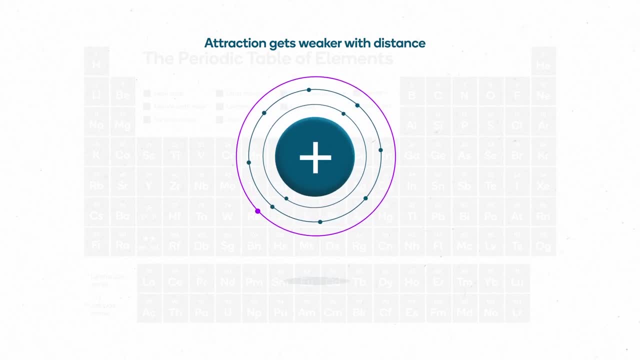 to its positive charge and this attraction gets weaker with distance, So as atomic radius increases. for the alkali metals, valence electrons are more easily lost to other atoms in a reaction. The really big alkali metals are called valence electrons: Alkali metal atoms like rubidium and cesium.